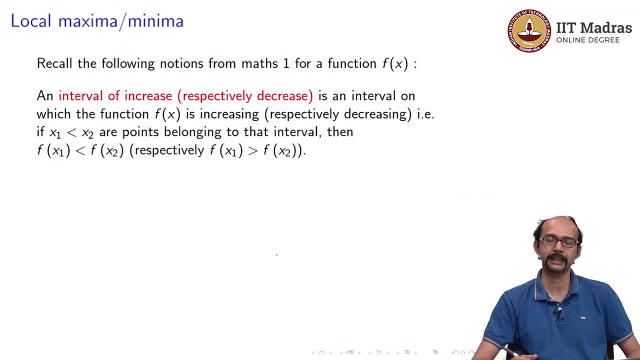 the function decreases from x1 to x2.. So f of x1 is greater than f of x2.. So these are notions that you have seen. I believe, in Maths 1.. We also saw in Maths 1, what is the turning point for a function. So point x is a turning point of fx, where 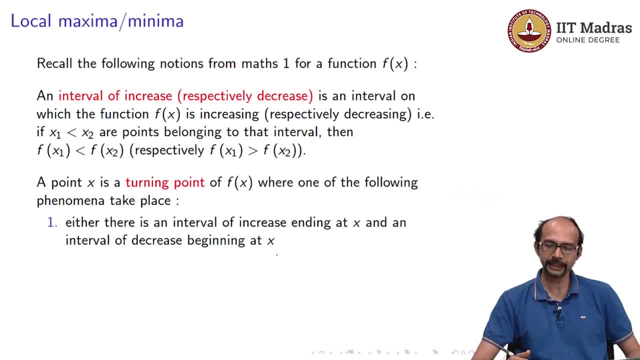 one of the following phenomena takes place: Either there is an interval of increase ending at x and an interval of decrease beginning at x, So that means the function decreases- sorry, increases till x and then decreases from x. There is some interval, So it need. 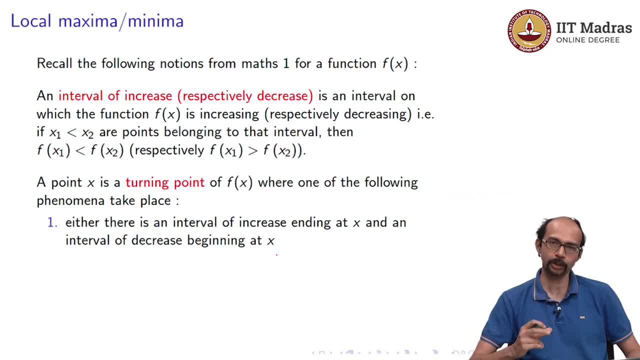 not increase throughout till x, but there is some small interval- could be small, could be large- which ends at x, and then from x there is again another interval which begins and in that it decreases, Or there is an interval of decrease ending at x and an interval of 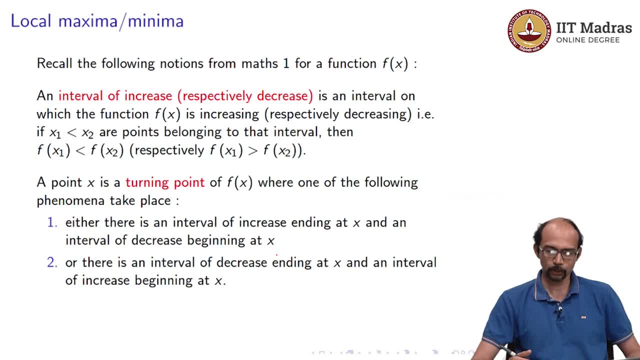 increase, beginning at x. So we will draw pictures of these in a minute, But I am going to give you some new names to call them by. So this is the definition which was in the title. A turning point, as in 1 above So 1 is this phenomenon, 1, which is to say the function increases till x, and 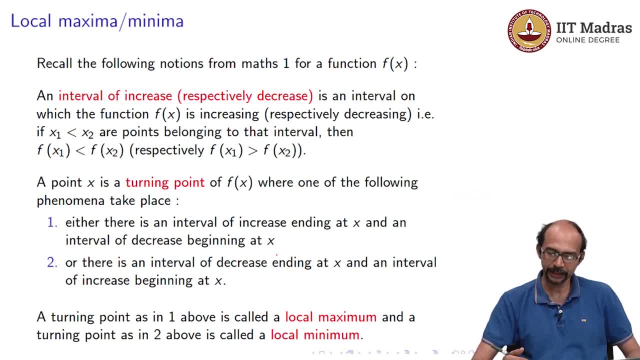 then decreases after x. So such a point is called a local maximum. That is because there is some some maximum interval you can be in which this on that interval. this point is where the maximum value of that function is attained And a local minimum is where you have phenomenon. 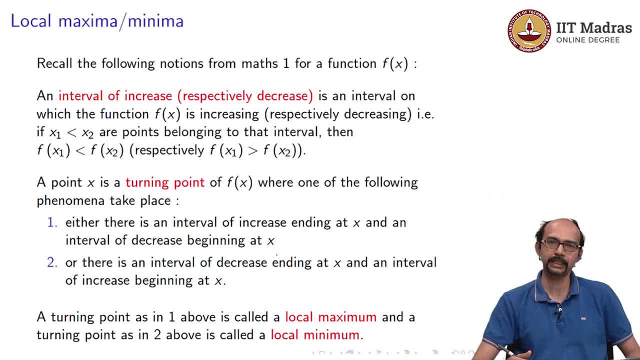 2 occurring, which means that first you have an interval of decrease and then you have an interval of increase. So the function decreases to x and then increases from x onwards. So let us look at this example. This is a very simple example. So the first interval 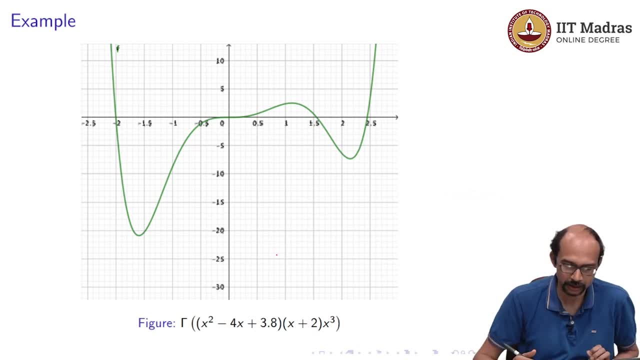 is the high end function and the second one is the negative. So this is the low end function example. So in this example we have plotted this function: x squared minus 4x plus 3.8 times x plus 2 times x cubed, what are the intervals of increase and decrease? So the 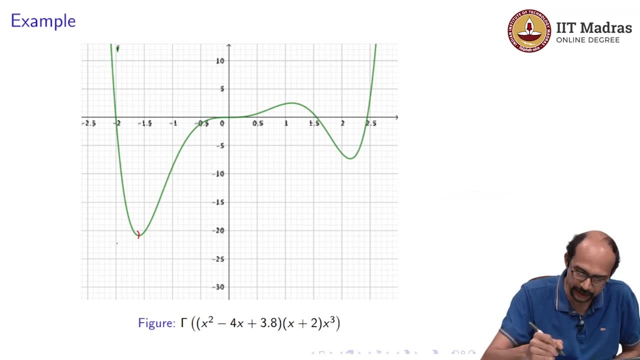 so until this point, this entire part, whatever is above here this is an interval of decrease, So decrease then after this, until you get approximately. here this is an interval of increase, although in the middle there is some strange thing happening close to 0.. And 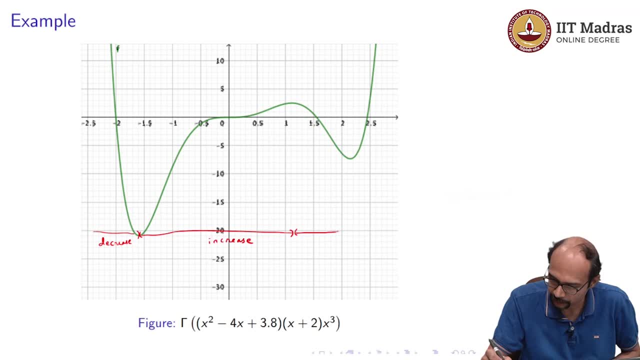 then, after this again, there is a interval of decrease till about here. So, and then after this again, we have increase, and probably increases all the way beyond this. So what are these points? So, in terms of what we have studied, what are these points? 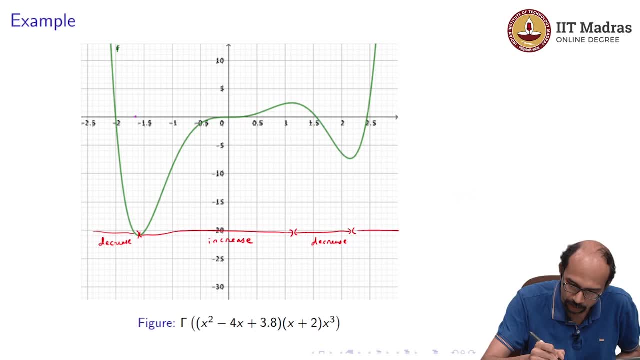 So this point here, this is a look some somewhere here, this is a local minimum for the function. and then this point here is another local minimum. So why is this a local minimum? You can see there is a valley here or a trough. 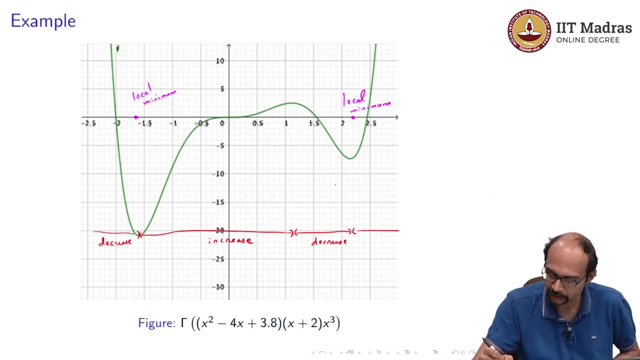 So if you choose some small interval, something like this, on this interval, the value taken by this point is the smallest. it is the minimum, So it is a local minimum. It is not, as you can see, it is not a global minimum, but this one actually looks like it is a global. 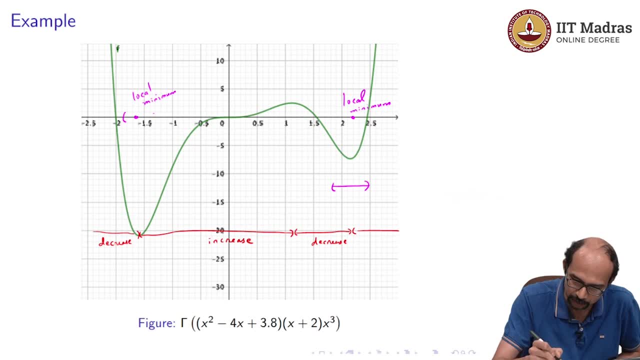 minimum. So here again you can choose some small interval, something like this: and it is a local minimum, meaning the smallest value on that interval, And in this case it so happens that it is actually a global minimum, meaning amongst all possible choices of fx. 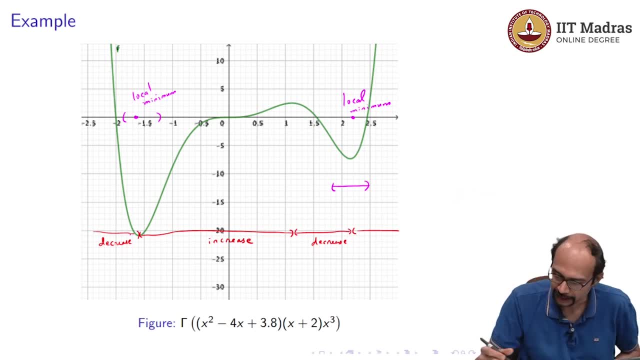 this is the smallest choice. And then what about this point here? That point is a, so that point is a local maximum. This shows you how these behave. and what is the interval here? Maybe you can take something like this, or you could have a larger interval. and it is. 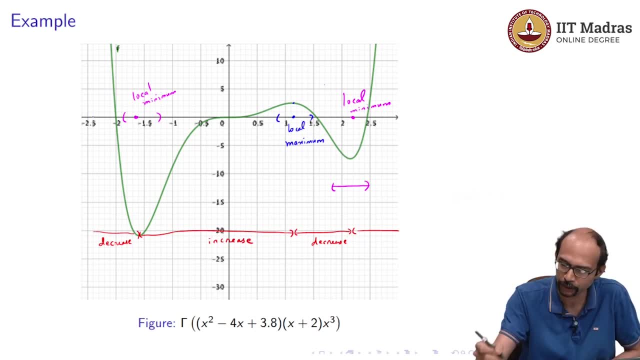 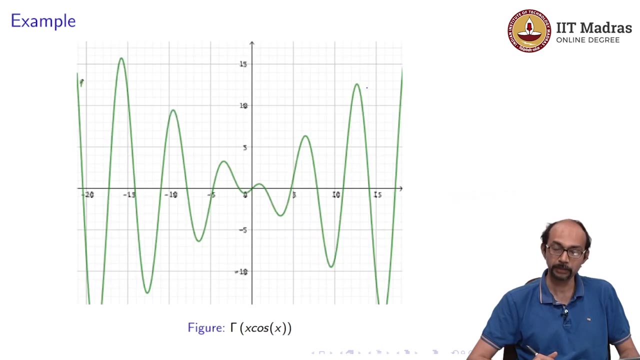 increasing. but you cannot say take this interval minus 2.5 to 2.5.. we may have values which are larger. In fact there are values which are larger. So I hope this picture is illustrative of the local minimums, minima and local maxima. 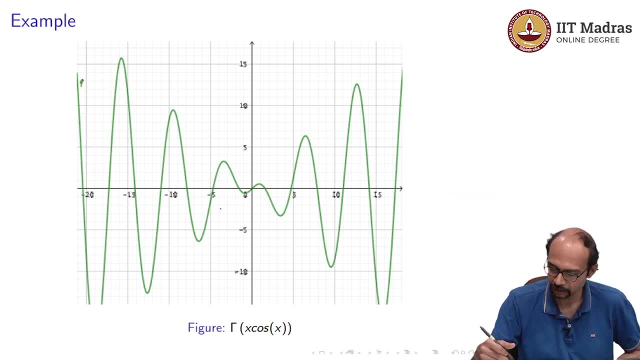 Let us do the same thing for this picture here. So this is the graph of the function x times cosine of x. And let us look at the local maxima. So here is one local maxima. So this point is a local maxima. this point here is a local maxima. 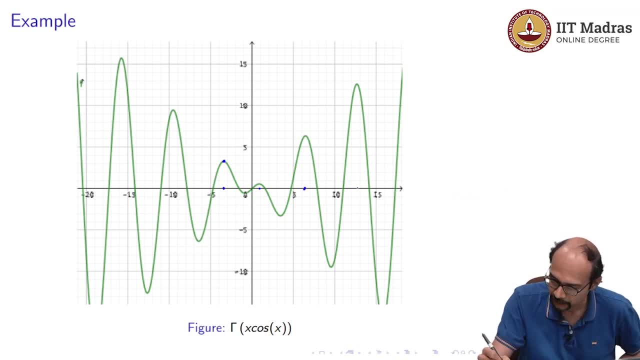 this point. here is a local maxima, maximum, local maximum, local maximum, local maximum, and so on. So this, since it is a nice wave like function with increasing amplitude, meaning with increasing amplitude, but a wave like, So you will have lots of local maxima, there will be infinitely many as you can. 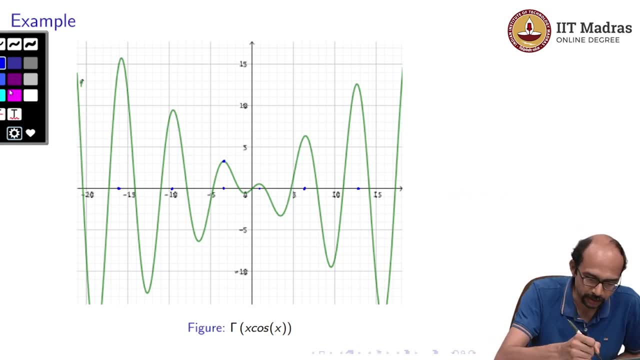 see, And what are the local minima? So let us also plot that. What are the local minima? Here is a local minima, local minimum. Here is another local minimum, local minimum. Well, somewhere here there is a local minimum. Here is one, here is one. 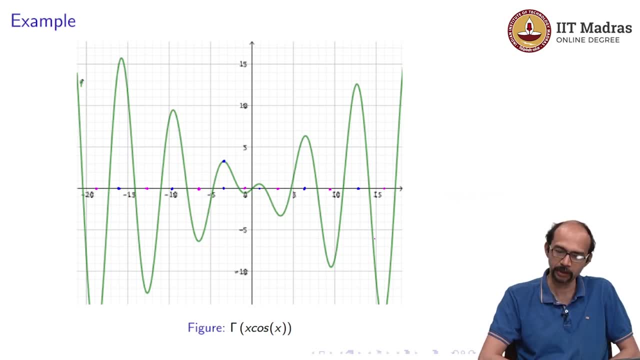 And somewhere here we cannot see the function value, but it is a local minimum. And the same thing happens as for the maxima. there are infinitely many local minima, So a local extremum is either a local minimum or a local maximum. 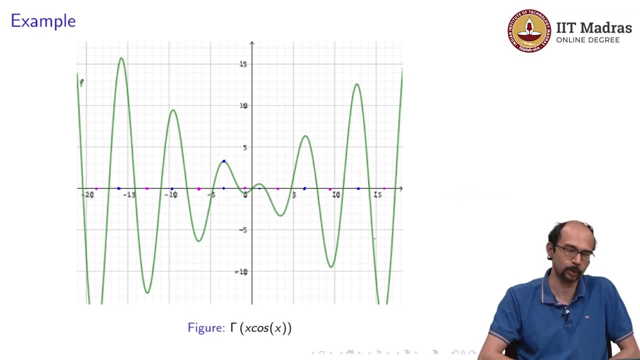 because it is an extreme value for in a small interval around that point, And often what we want to do is to ask: how do we find these local extremum? So these values are they often have, they are turning points And they are also the turning points for the maxima And they can be. 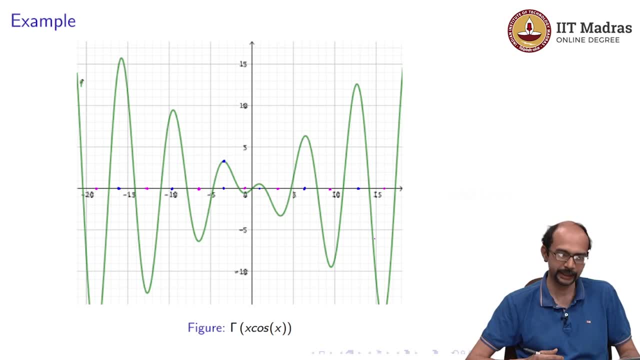 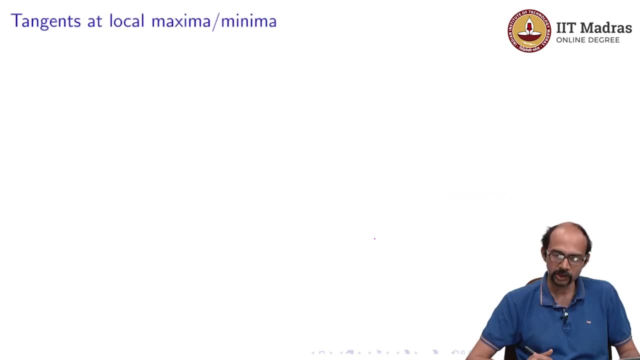 and they often carry information about the function with them. So often we want to ask, we want to study how to find them. So one way that we can think about to find them is to look at the tangent. So we have been studying tangents for a while now, and this is another. 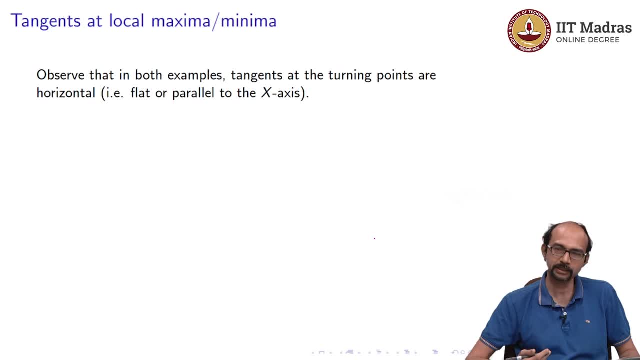 application of tangents. and well, once we have tangents, you know now what is going to come. but let us hold on to that idea for a minute. So observe that in both examples tangents at the turning points are horizontal, So they are flat or parallel to the x-axis. So 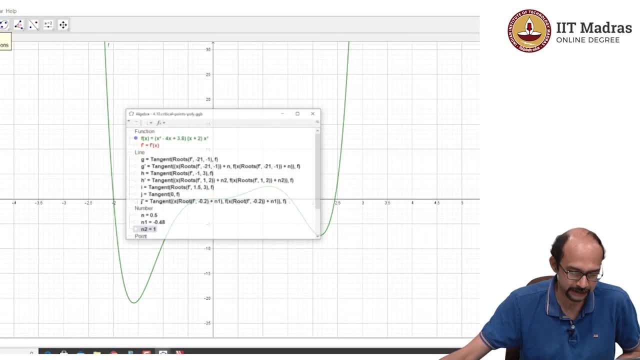 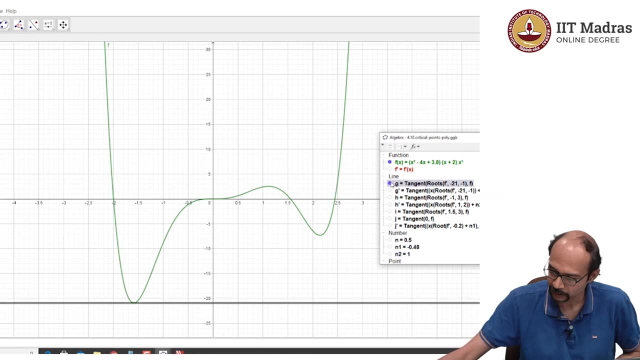 let us look at the first example. let us look at what are the tangents at these various points. So if you look at the tangents at the various points, well, let us look at this tangent well, you can see it is parallel to the x-axis or it is horizontal. 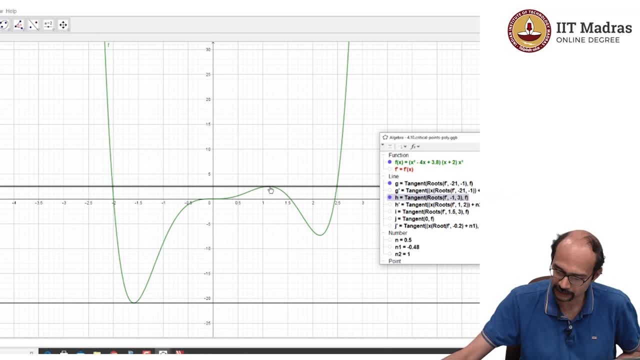 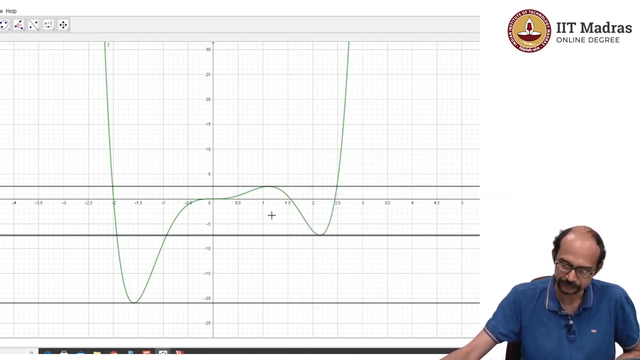 Here is the tangent to this local maximum. it is again horizontal. And let us look at the tangent to this local minimum here. that is also horizontal. So these were the 3 points that we identified as local extrema in this case, and all 3, the tangents are horizontal. 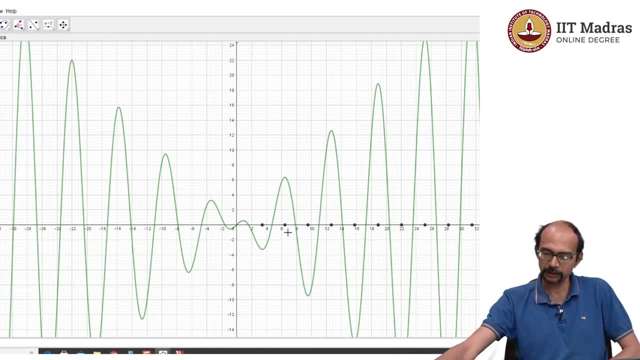 Let us look at the other picture. So it is clear that that these points, if you draw the tangent over here, it will be a local, sorry, it will be horizontal. So at this point, or this point here, or this point here, So at all these. 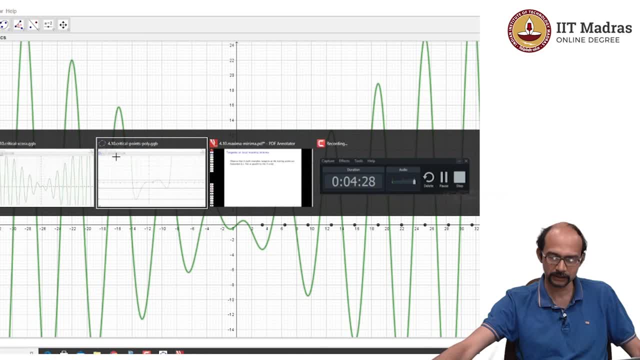 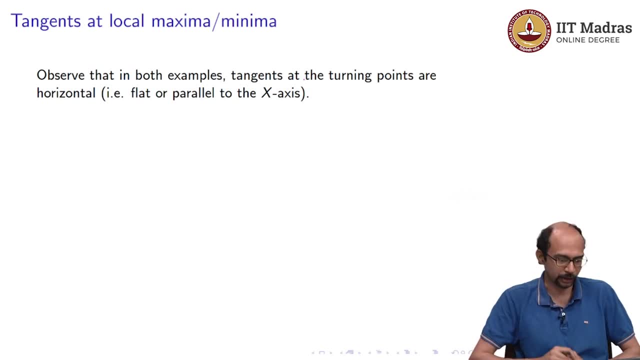 points they are going to be horizontal. So I think at least the picture is very clear and unambiguous in telling us that at turning points the tangents are horizontal. So this is a general phenomenon, that it is easy to visualize this, and let me just draw. 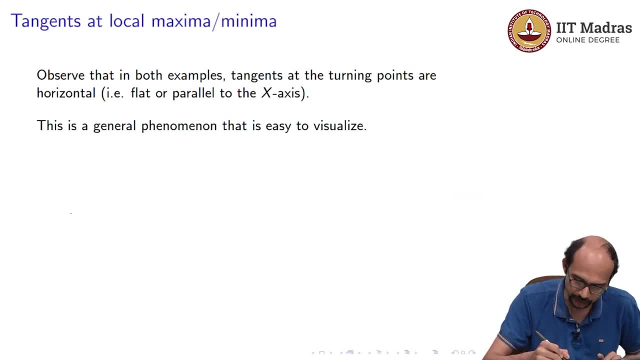 this picture so that we have an easy way to visualize this. So, if you have a local minimum, it is going to be something like this: If you have a local maximum, it will be something like this: And now, how is the tangent going to look like? So, if you draw the tangent, 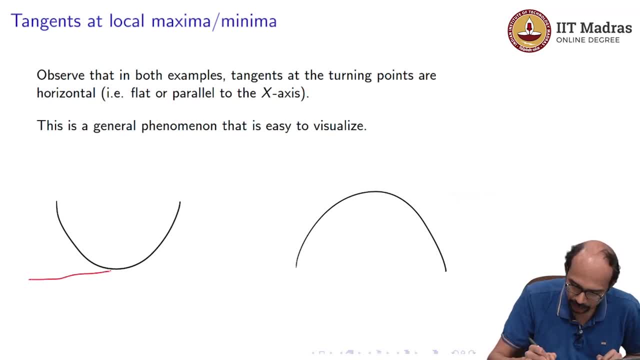 the tangent to this thing over here, it will look like this: the tangent to this thing over here will look like this. So you can see it is horizontal, although it is not very well drawn, So it is something that is easy to visualize. So, but how do we make this? 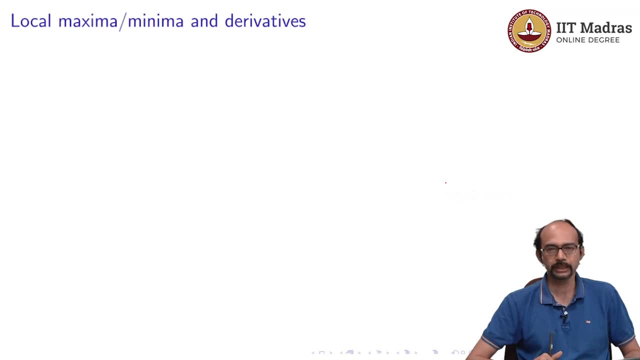 formal. So the way to make it formal is to, of course, introduce derivatives, as we have been doing for a while now. we have been capturing the idea of tangents in terms of derivatives, and so derivatives give us an algebraic way of getting hold of equations and so on. 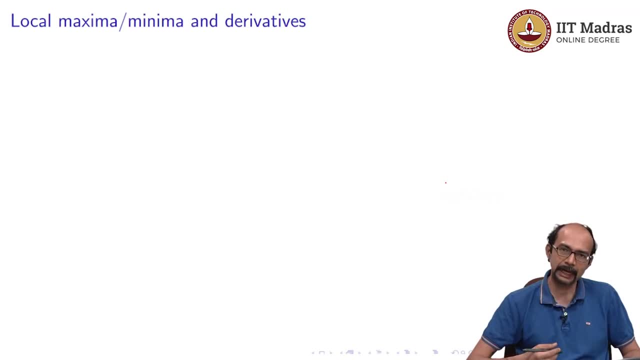 And that tells us how to. that will help us in analyzing how to first prove that the tangent will be horizontal and, second, to utilize it for further study of local maxima and mean. So how do we prove that the tangent, if it exists? note that tangents may not exist in. 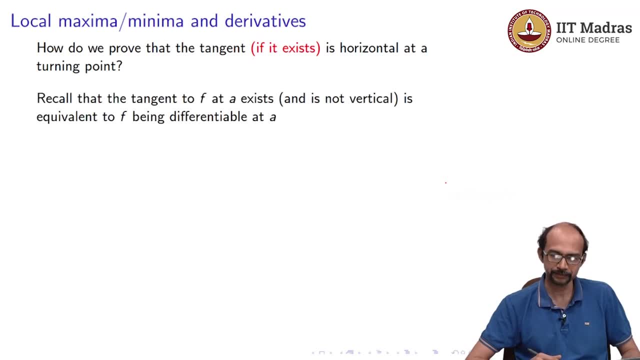 general. So if it exists, So if it exists is horizontal at a turning point. So recall that the tangent to f at a exists and is not vertical- is equivalent to f being differentiable at a. This was something that we observed in our previous video And in fact we know how its equation looks like. 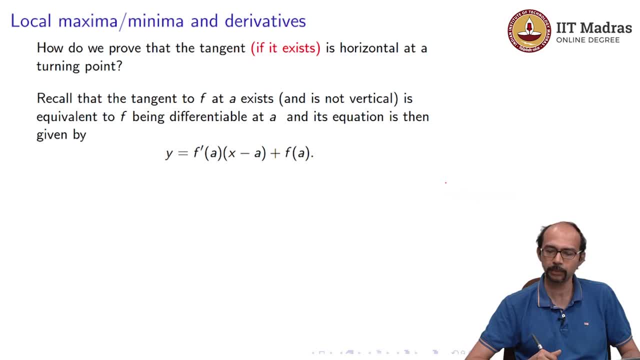 Its equation is then given by y: is f prime a times x minus a plus f of a. So proving that the tangent, if it exists, is horizontal at a turning point is equivalent to showing that f prime a is 0.. So let us show that f prime a is 0 on turning points. So if a 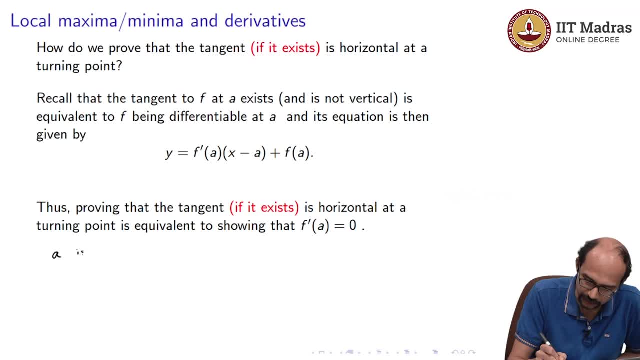 is a turning point. so a is a turning point and f prime a exists, So that of course we cannot guarantee, but assuming that is the case, Okay, Okay, Let us show that f prime a is 0.. So suppose, just for the sake of argument that we have, 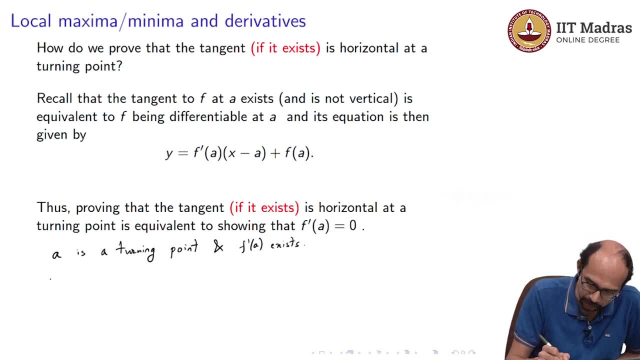 a local maximum. So suppose a is a local maximum. So what does that mean? That means that for h greater than 0, there is some small interval, or maybe I should first say that is a. So for some open interval, a comma, or maybe not a, a minus. 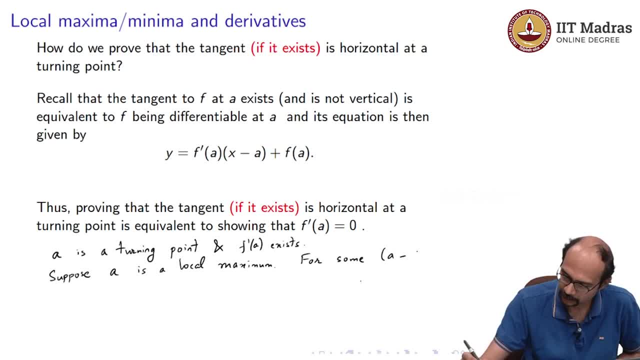 a Yeah. So for some open interval, a comma, or maybe not a, a minus a. So for some open interval, a comma, or maybe not a, a minus a, some small number, let us call it epsilon. So for some a minus epsilon comma, a plus. 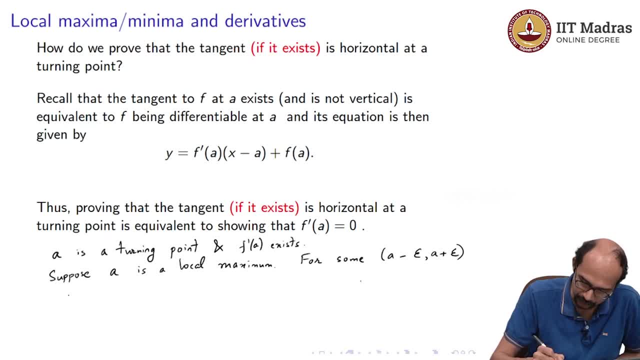 epsilon. if h is less than epsilon, then f of a minus h is less than f of a, and f of a plus h is less than f of a. That is when you will say that this is a local maximum. So now let us apply the definition of the derivative. So f prime, a is limit, h tends. 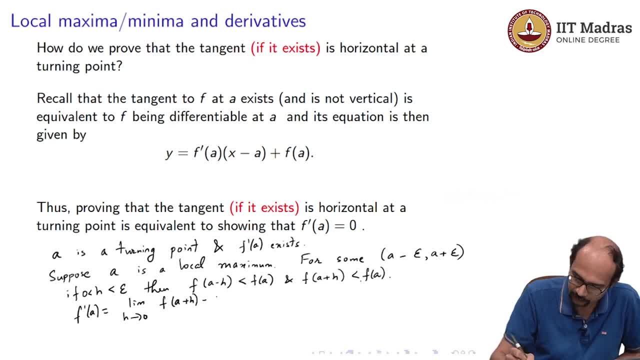 to 0, f of a plus h minus f of a divided by h. But notice what happens to the numerator when you have h is between 0 and epsilon, So f of a plus h is less than f of a plus f of a. So this numerator is negative. So this value is going to be less than or equal. 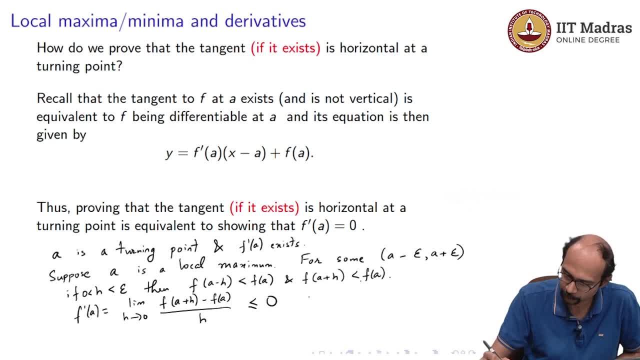 to 0.. So this is the derivative from the right. So this is limit h tends to 0 plus. So this is going to be negative. On the other hand, we know that f prime a is also equal to limit h tends to 0 minus. 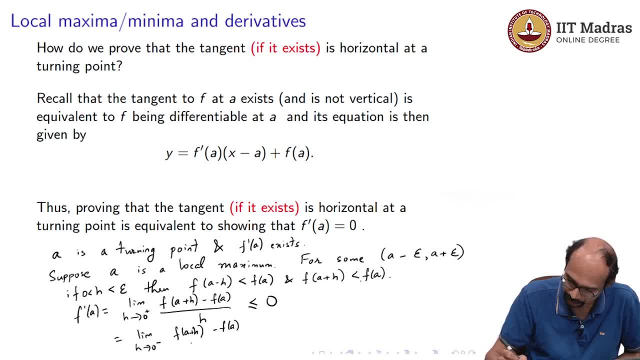 f of a plus h. So this is going to be negative. So this is going to be negative. So this is f of a divided by h. So here, of course, h is between minus epsilon and 0. So in that, 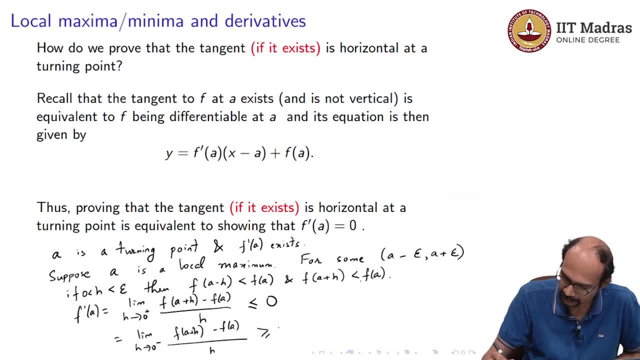 case this is going to be greater than or equal to 0. Why is that? Because here the numerator is negative, but the denominator is also negative. So negative by negative gives you a positive number. So now we know that f prime a exists and it is greater than. 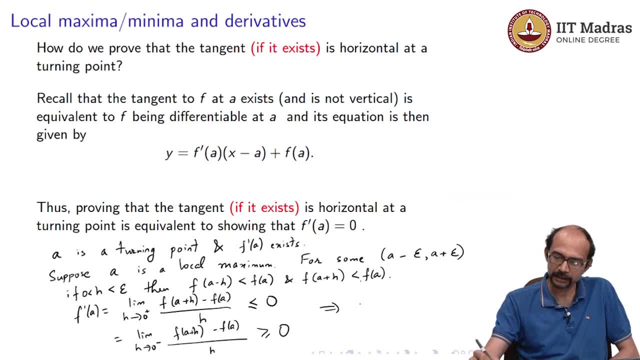 or equal to 0, and we also know it is less than or equal to 0, that tells us that f prime a must be equal to 0. So you can see the power of the left limit and the right limit coming in here. So if it is a turning point, then f prime a must be 0, f prime a is 0 is. 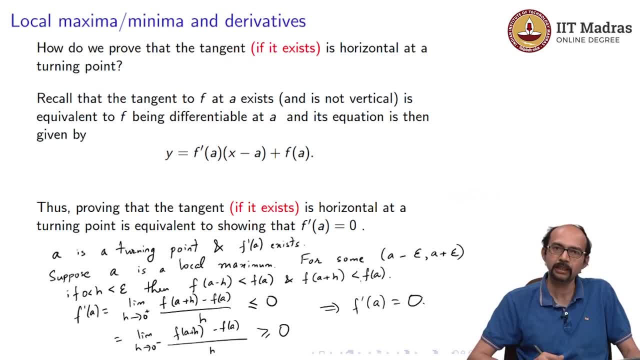 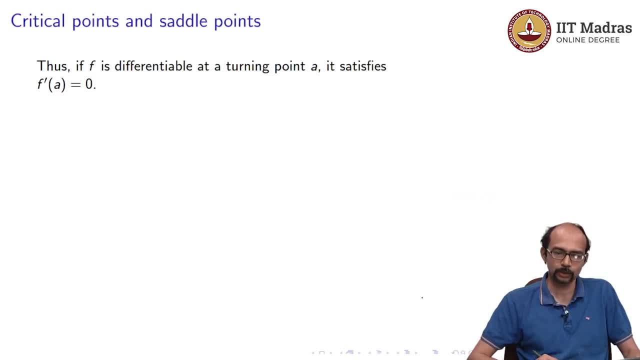 exactly the same as saying that the tangent is horizontal or parallel to the x axis. Okay, So we have actually proved that. So let us now ask how we can harness this information to actually study turning points. If f is differentiable at a turning point, a, it satisfies. 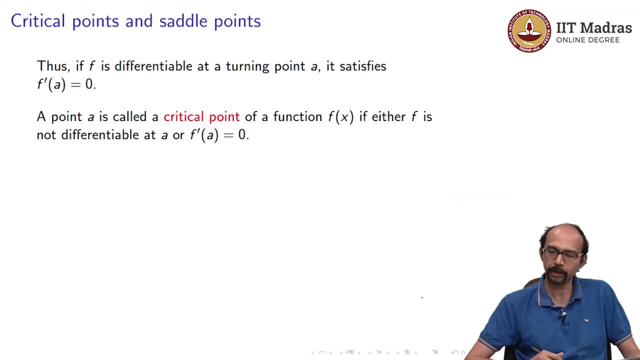 f prime a is 0. So point a is called a critical point of a function f, if either f is not differentiable at a or f prime of a is 0.. So either it is a point at which the function is not differentiable or it is differentiable. 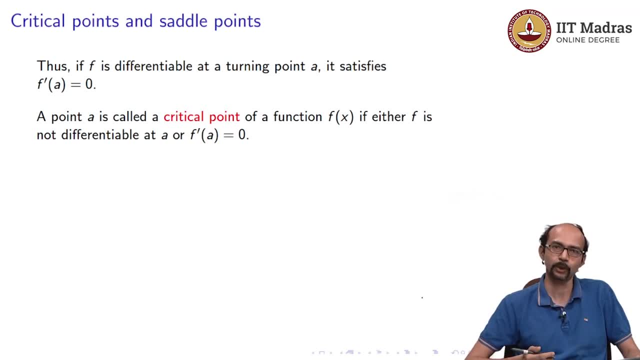 So f prime a is 0 if it is differentiable, and when you take the derivative, the derivative is 0 at that point. So of course every turning point is a critical point. we just saw that if you have a turning point and f prime a is 0 if it is differentiable, and if it is, 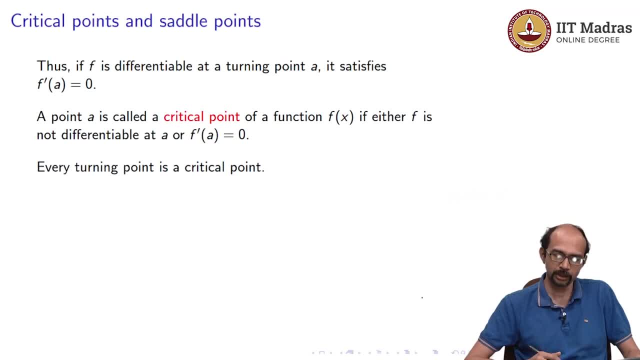 not differentiable, it is a critical point anyway. So thus, in order to find turning points, which is to say local maxima or local minima, we will first find critical points. So suppose f is differentiable, So is every critical. 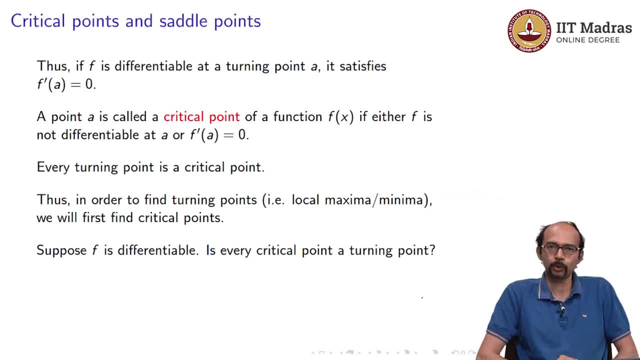 point, a turning point. So what do we want to do? We want to find turning points. So that is local maxima or local minima. By the way, I should point out that the plural of maximum is maxima and the plural of minimum is minima. 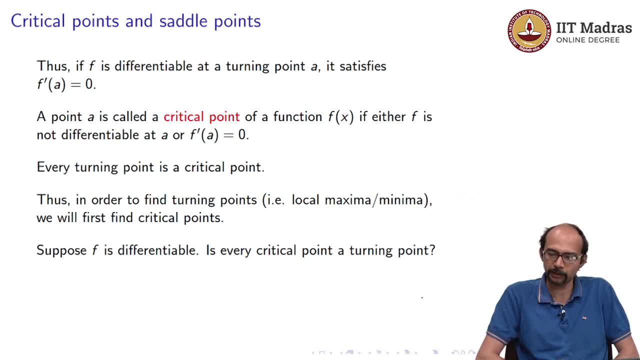 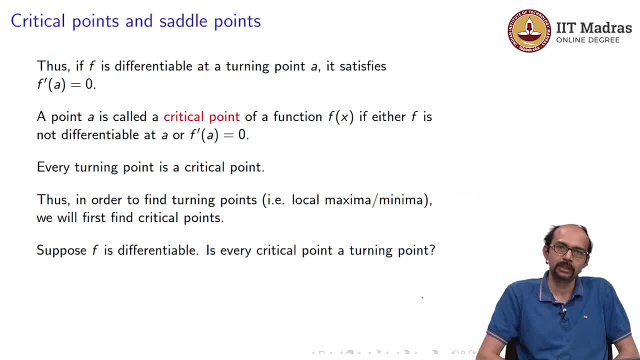 sum will be local minima, But are there any others? That is the question. So is every critical point a turning point? So, if there are no others, we really have the entire set of local maxima and local minima just by finding the set of critical points. 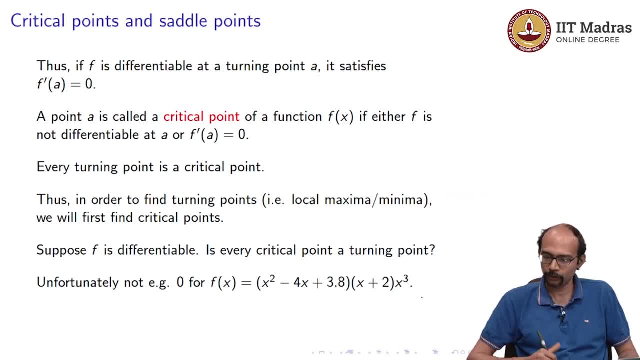 So unfortunately that is not the case. So if you look at that function that we had earlier- x square minus 4x plus 3.8 times x plus 2 times x cube- and we look at the value 0,, 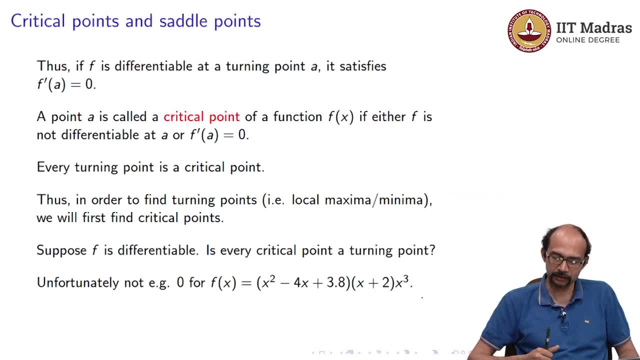 then we can see that it is going to be a critical point. So I will just make this definition. So a saddle point is a critical point which is not a local maximum or local minimum. So I want to make a small caveat. 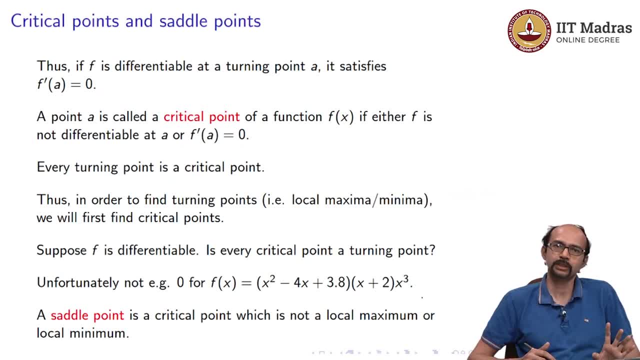 Here. somehow different sources use different names for this. So saddle point is common. when we go to beyond one dimension, which we will do in subsequent weeks, In one dimension there are different words used. some people seem to use the word inflection point, So 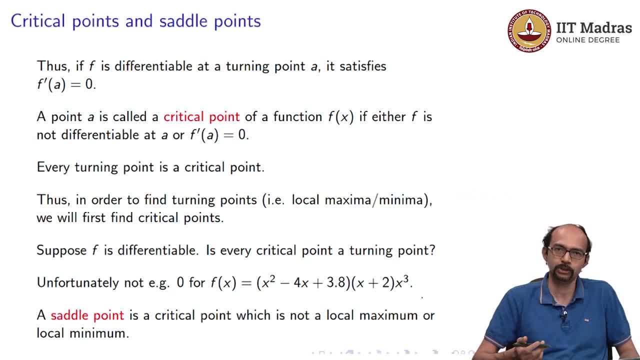 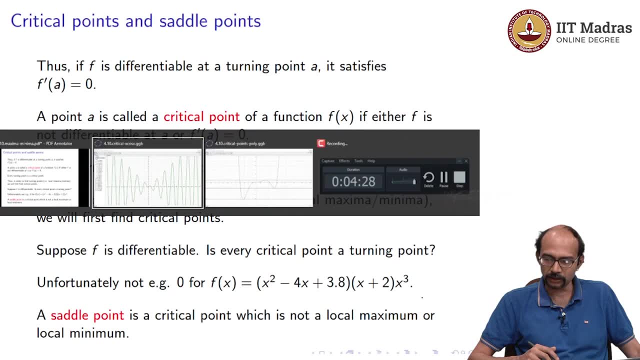 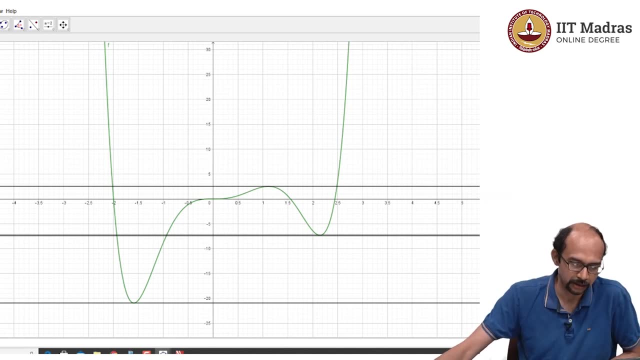 be careful of. depending on the source that you study, they might use a different word for this. So let us look at the picture of this function. So here is the function that we had: f of x is x square minus 4x plus 3.8 times x plus 2 times x cube, and let us draw all the points. 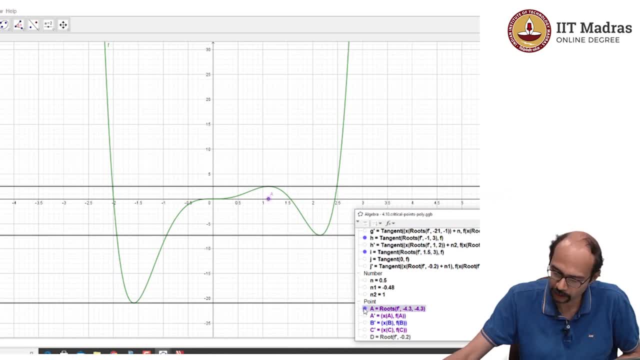 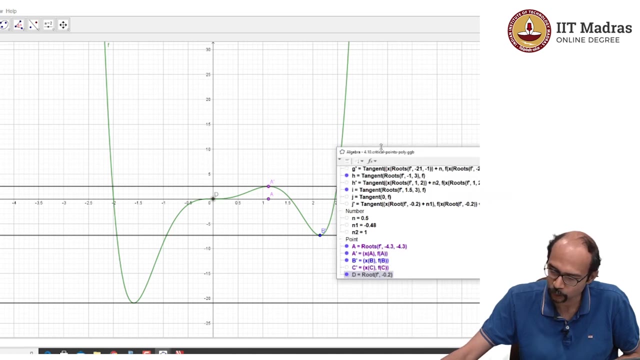 So here is one of the. here is the local maximum of the set of critical points. So, and maybe corresponding to that local maximum, we have the corresponding value. Here is your local minimum, the point B prime, and here is the point 0, 0, which is a saddle point. 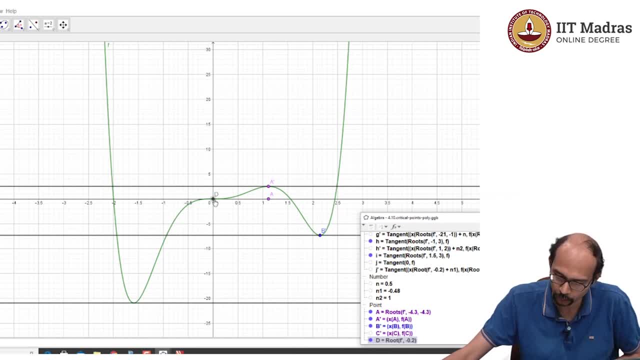 Why is that? a saddle point, As you can see, as if you draw the tangent to this point, tangent to f at this point, let us draw the tangent Here it is. So, if you draw the tangent, it is actually the x axis, and you can check this by writing down the equation, So you 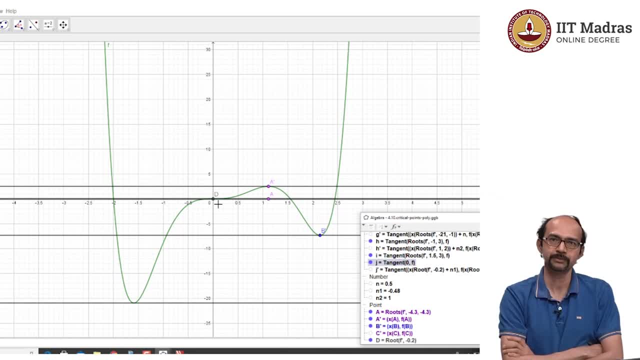 have an x cube in the expression. So if you differentiate the function, we will obtain that f prime of at 0 is going to be 0. So the it is a good exercise. Okay, So this is actually to do that. So, and there is also a point here which unfortunately, 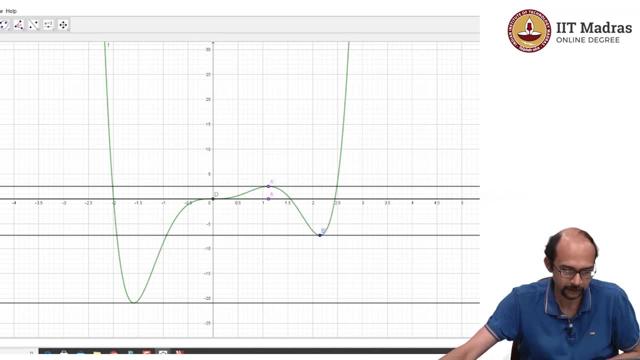 has not gotten marked This and that corresponding number somewhere here. So this is a local minimum, the corresponding point here is a local minimum, the point A is a local maximum and D is a saddle point. So I hope now we have done all the critical. 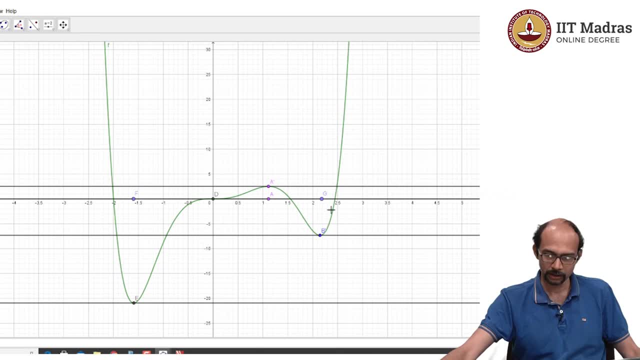 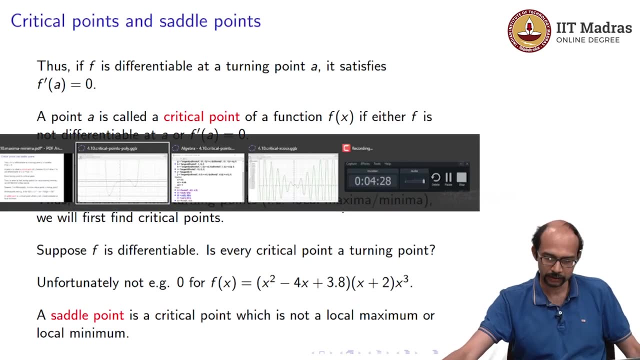 points of this in this picture. So I hope that it is clear what a saddle point is. So just to again reiterate what is happening for a saddle point: So this is a saddle point. You can see that for a saddle point there is something special happening. It is not. 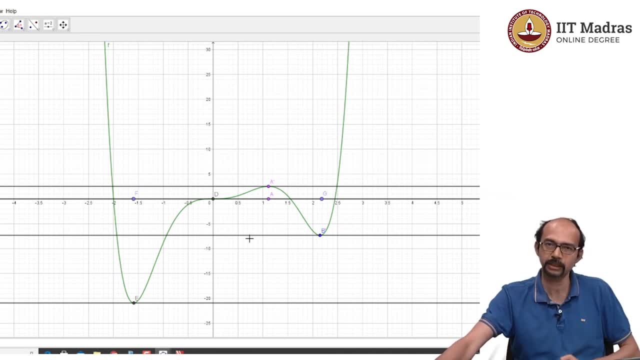 a local minimum or maximum. but the function behaves in a slightly weird way. So it is concave below before it hits that point and it is concave above after it hits that point. So between E and D it is concave below and between D and A it is concave above. 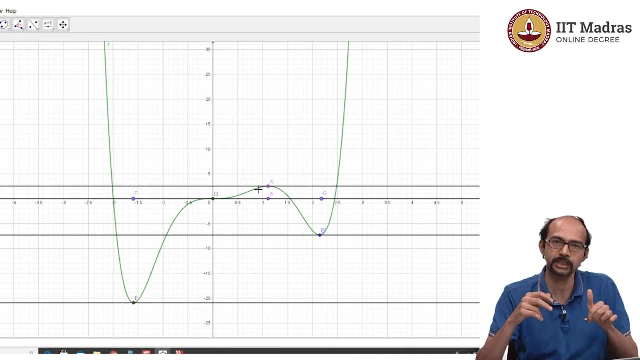 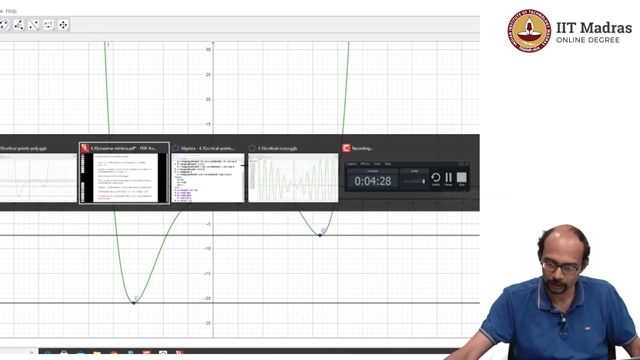 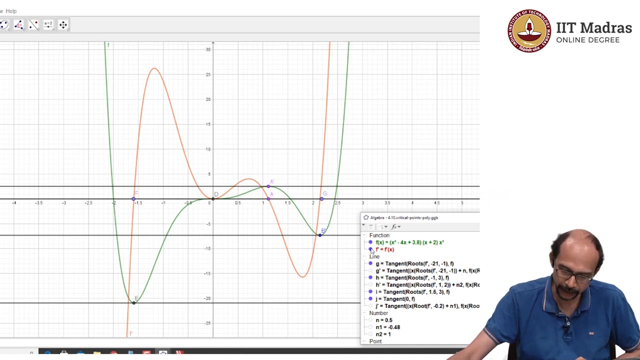 So there is something happening, there is some change which occurs, and that change is really what is reflected by this point. And whenever such a thing occurs, such points are going to be critical, are going to be saddle points. So let us also draw the f prime. So this is f prime. So if you 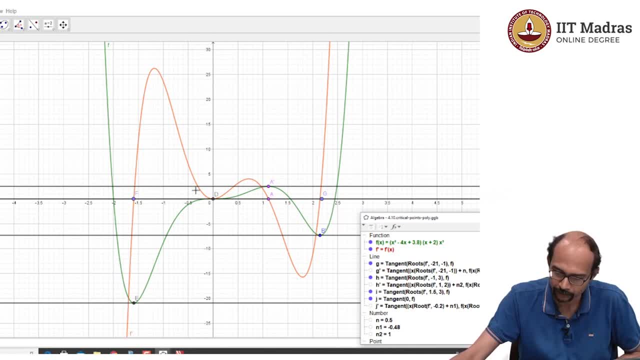 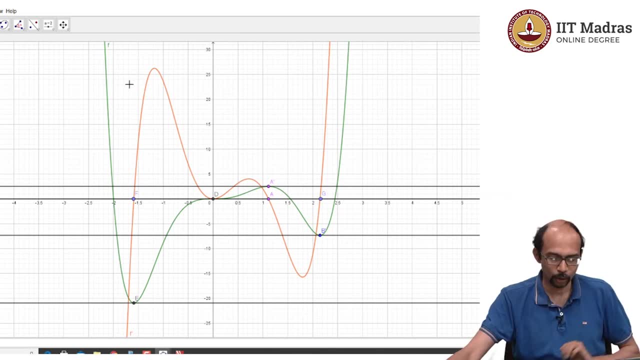 look at f prime. these are exactly the zeros of f prime. f is a 0, D is a 0, A is a 0 and so this point G is a 0. So we have identified all the critical points correctly for this function. 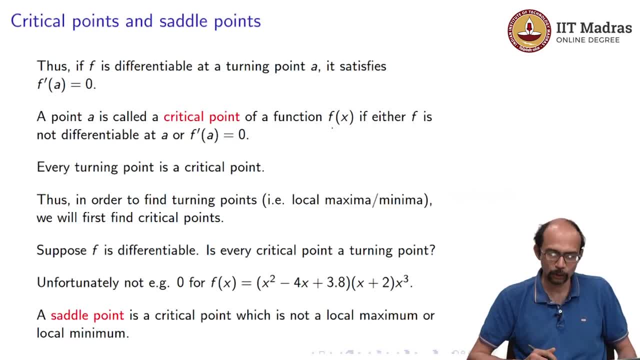 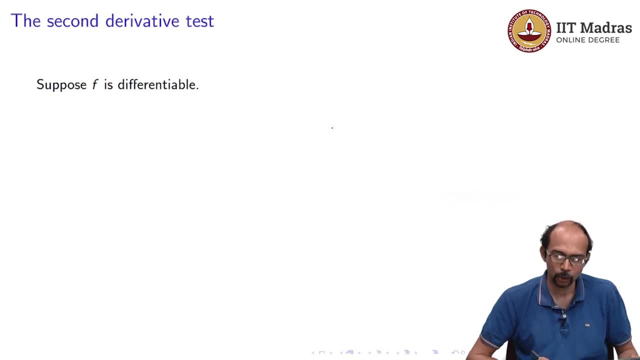 So let us go back to our slides. So I hope in this example it is clear what is a saddle point and what is what are the local maxima and minima? So now, how do we find out of these critical points? how do we find which ones are local? 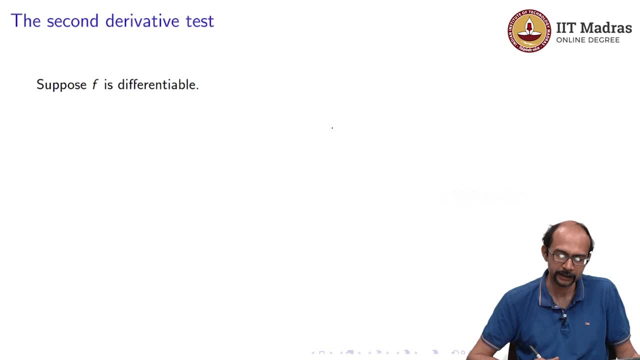 maxima and local minima. Those are the ones that we want to find. So let us assume that the function f is differentiable. How do we classify critical points? So we use the second derivative test. So, just like the first derivative f prime checks for the monotonicity of the. 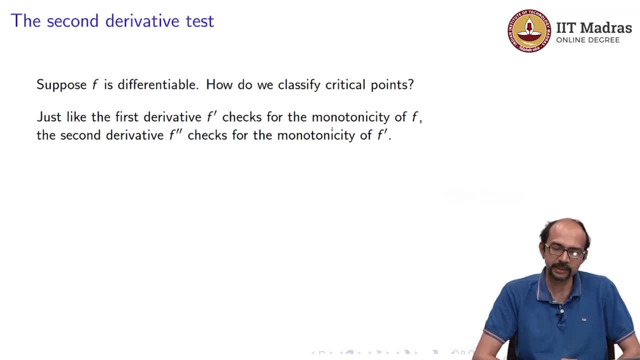 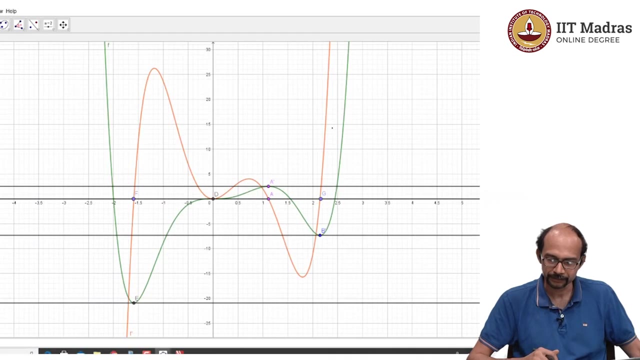 function f. that is what we saw. The second derivative, f double prime, checks for the monotonicity of f prime And based on this monotonicity we can see how the behavior is. So let us go back to our picture. So here is our picture for f prime. 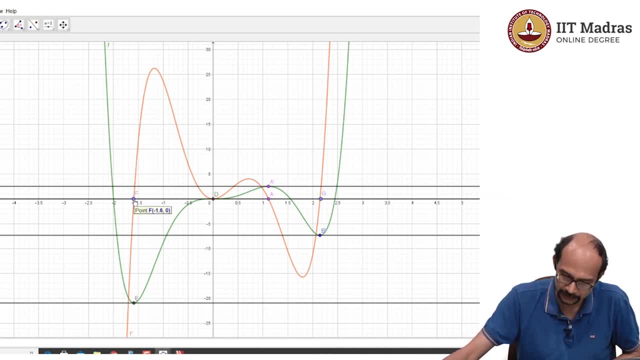 And you can see that for the point f it is a 0 of this function, f prime, but this function is very nicely increasing at f. And similarly for the point A the function is 0 at that point A but the function is decreasing for that point A. 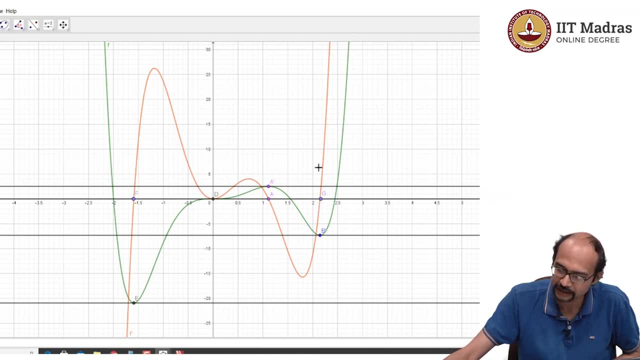 And similarly for the point G, the function is increasing at that point G. But for D this function is behaving in a totally different way, Namely: if you, this function is a, so D is actually a local minimum for the derivative. 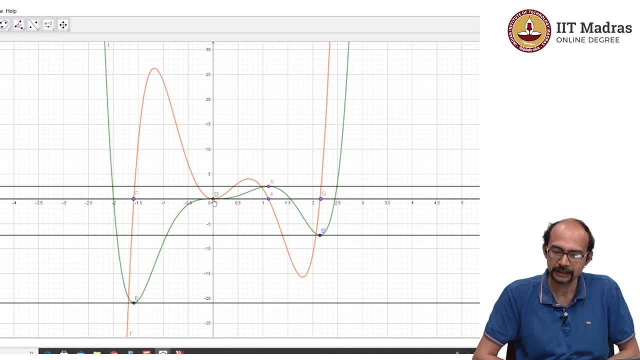 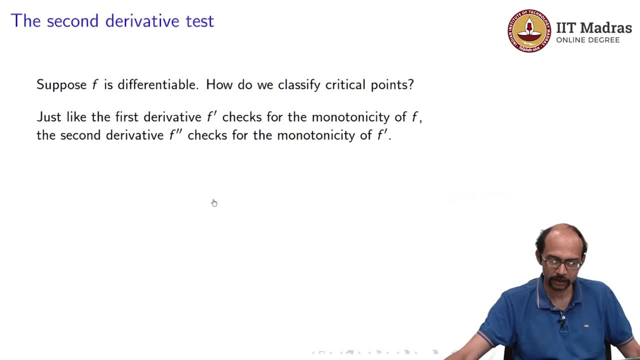 So. so when such a thing happens, that is going to be a critical point or, sorry, that is going to be a saddle point. So let us see what is the second derivative test. So the second derivative test is the following: So if f is twice differentiable, 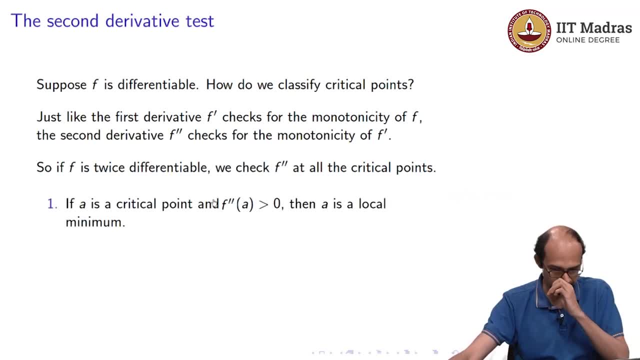 we check f double prime at all the critical points. If A is a critical point. if f double prime A is greater than 0, then A is a local minimum. If A is a critical. if f double prime A is strictly less than 0,, then A is a local maximum. If A is a critical point. 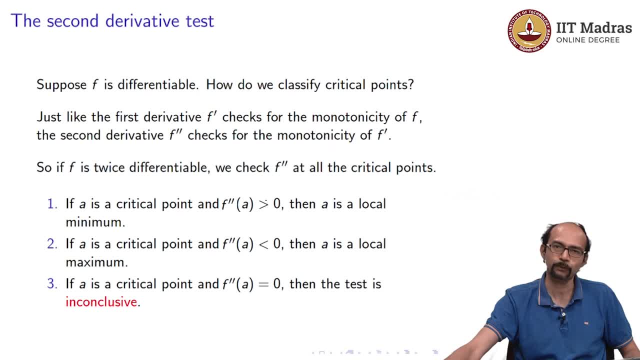 if f double prime A is 0,, then the test is unfortunately inconclusive And that is a little sad that there is. this is not a absolute test And we will see why that is the case later on. So let us quickly conclude. 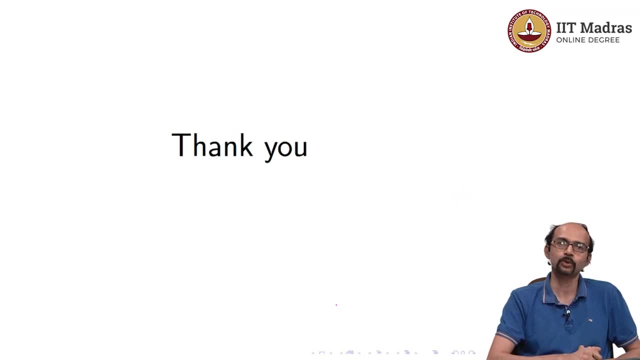 by recalling what we have done in this video. So we have checked how to obtain critical points That when you put the derivative to 0 or if the function is not differentiable at the point, Assuming that the function is differentiable and in fact twice differentiable-